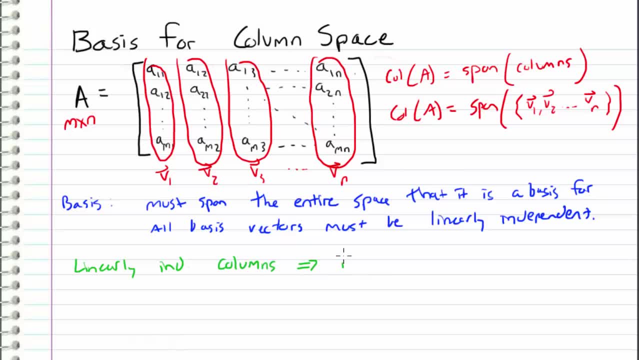 columns are just the pivot columns. So what this means is the pivot columns form a basis for the column space. Now for that, in order to calor folding cosmos, follow 2tober to theерб of step 4 and f to space of our matrix. so, in order to find a basis for the column space, it's just a. 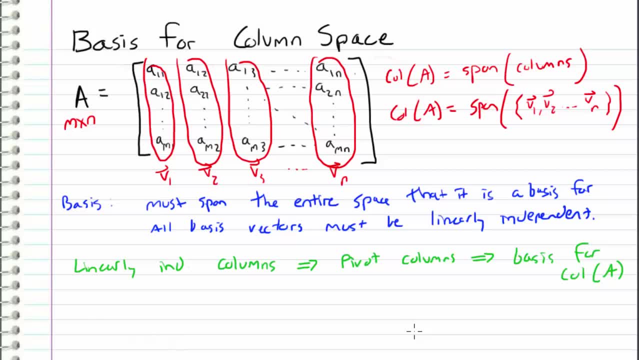 matter of picking out the pivot columns of that matrix. and since the non pivot columns are linearly dependent with the pivot columns, then we can say that the span of all of the columns is equal to the span of the pivot columns, and from this fact up here we know that this is equal to the column space of a. therefore, 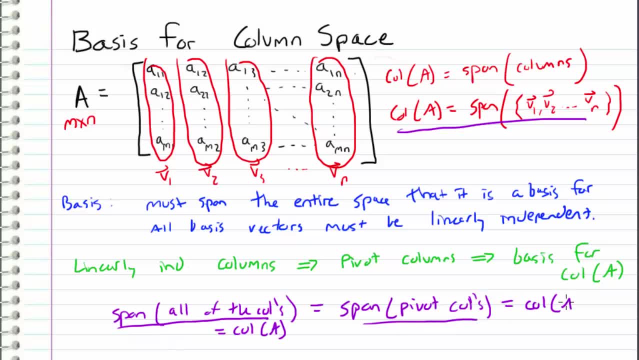 this must also equal the column space of a. so that means that the span of the pivot columns is equal to the column space of a. so it satisfies this criteria for a basis and also, since the pivot columns are all linearly independent, it also satisfies this criteria. so that's why we use the pivot columns of a matrix. 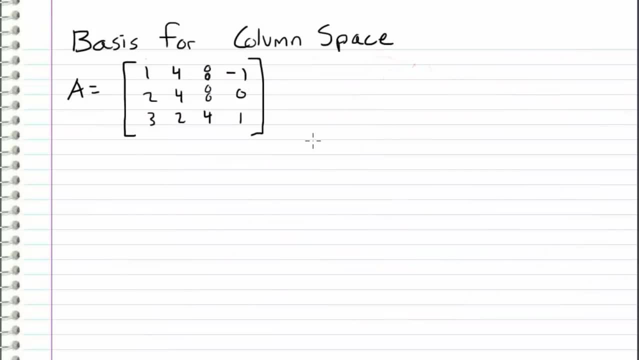 to be the basis for the column space of a matrix for the column space. so here's an example that we're going to take a look at. we have a matrix a that is equal to 1, 2, 3, 4, 4, 2, 8, 8, 4 and negative 1, 0, 1. so we 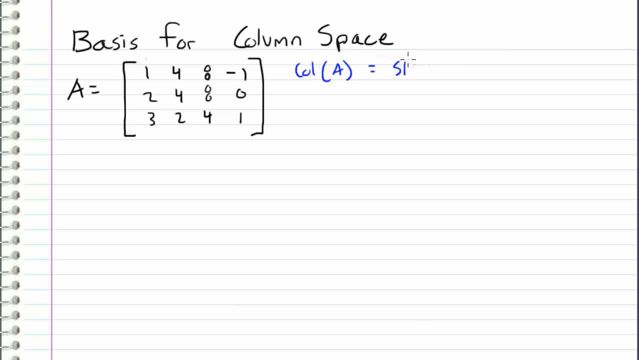 could say that the column space of this matrix is just the span of the vectors 1, 2, 3, 4, 4, 2, 8, 8, 4 and negative 1 0, 1.. So now what we want to do is we want to find a basis for this column space, or in: 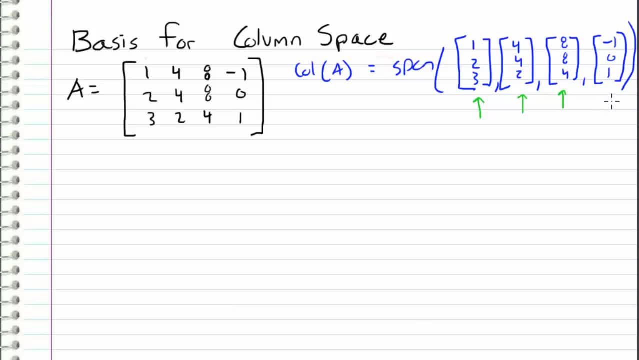 other words, we want to look at each of these vectors and figure out which of these are linearly independent, and we want to eliminate the linearly dependent vectors. and once we filter out the linearly deep in in vectors, what we're left with is a basis for the column space. so the first thing that I need to 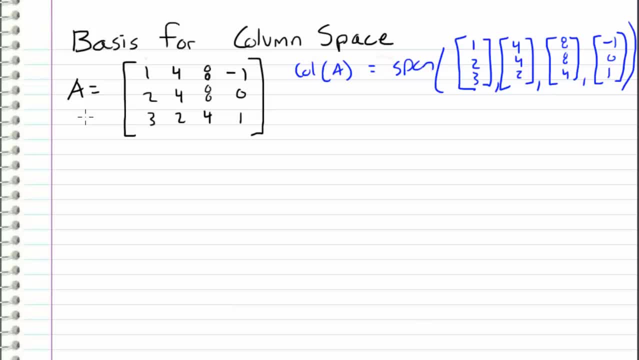 do in order to identify the pivot columns is first identify the pivot locations, And in order to do that, I need to reduce this matrix into its row echelon form. So we'll perform Gaussian elimination on this and we'll use this as the first pivot. 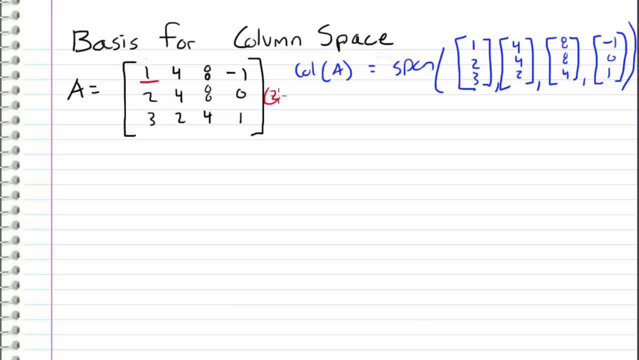 and we're going to eliminate everything below it. So, in order to do that, we can take the second row and subtract 2 times the first row, and we can take the third row and subtract 3 times the first row, And what we're left with is a row equivalent matrix 1,, 4,, 8, negative 1,. 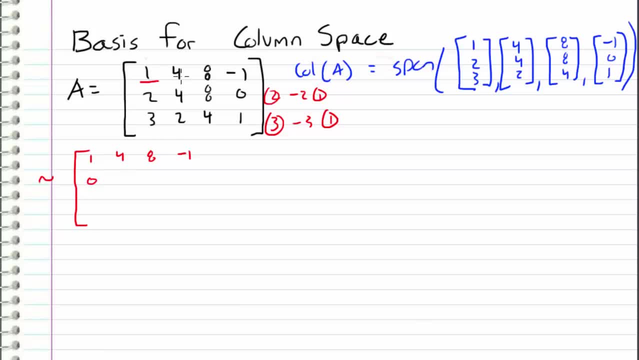 and then we have 2 minus 2 times 1,, which is 0.. 4 minus 8, which is negative 4.. 8 minus 16, negative 8.. And 0 minus a negative 2,, which is positive 2.. 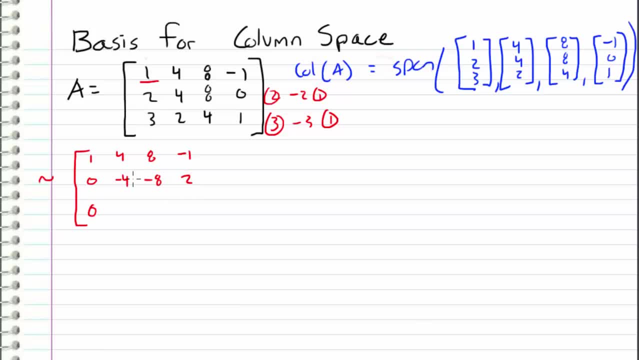 And then in the third row, we have 3 minus 3,, which is 0.. 2 minus 12,, which is negative 10.. 4 minus 24,, which is negative 20.. And 1 plus 3,, which is 4.. 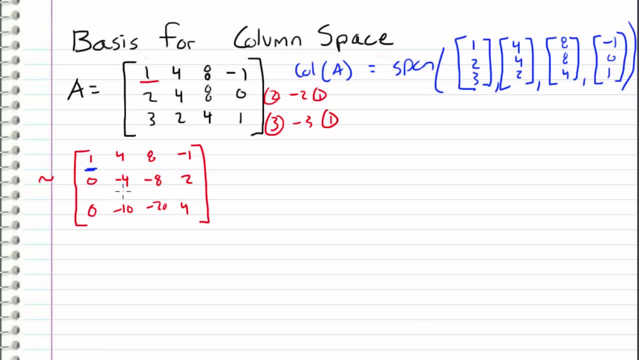 So, now that I've just used this as a pivot, I'm going to move on to the next pivot location, which is this guy, and I'm going to try to eliminate everything below it, And I can do so by taking the third row. 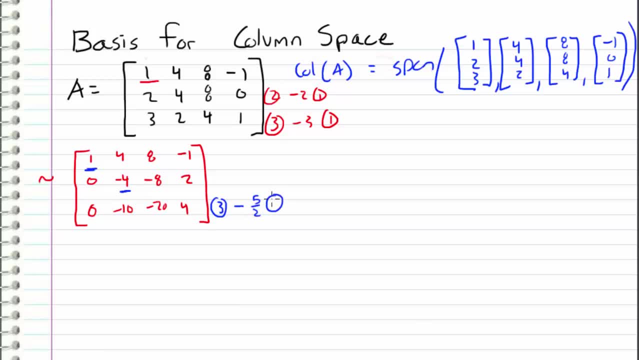 and subtracting 5 halves times the second row. So when I perform this operation I get a row equivalent matrix, where the first two rows remain the same And in the third row I have 0 minus 0, which is 0.. 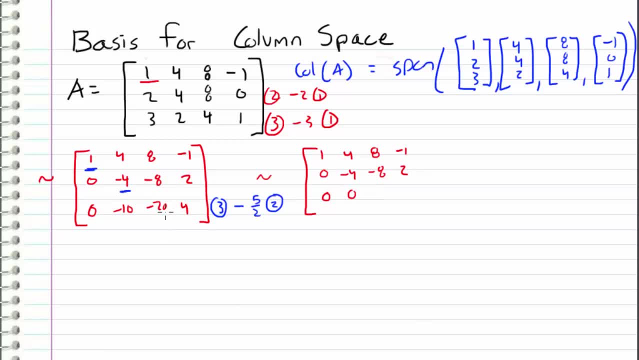 Negative 10 plus 10,, which is 0.. Negative 20 plus 20,, which is also 0.. And 4 minus 5, which is negative 1.. So we can recognize this matrix And then we can take the first row echelon form of our matrix A. 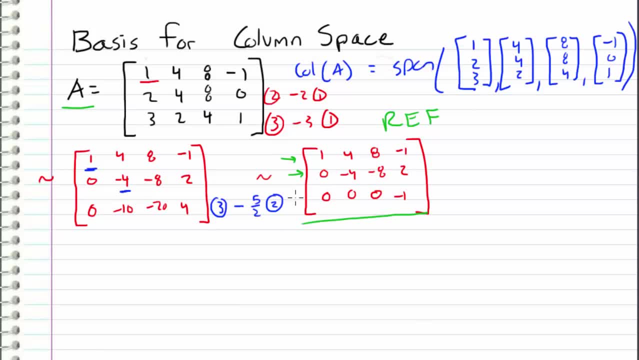 Therefore, we can look at the first non-zero entries of each row and we can pick out the pivots which are these guys right here, And then we could take the corresponding pivot columns, which correspond to the first, second and fourth columns. 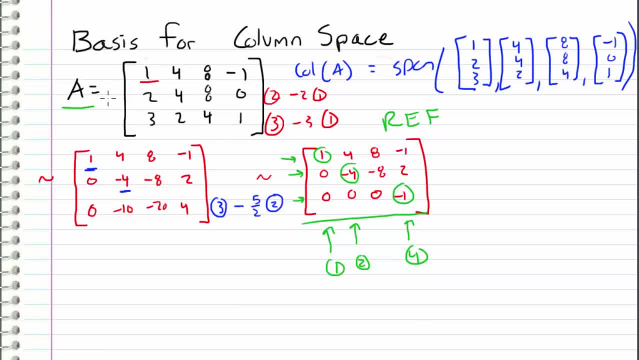 So what we do now is we go back up to our original matrix and we select the first, second and fourth columns, And these columns that I just circled in green are the pivot columns of our matrix And therefore we use these pivot columns as the basis for the column space. 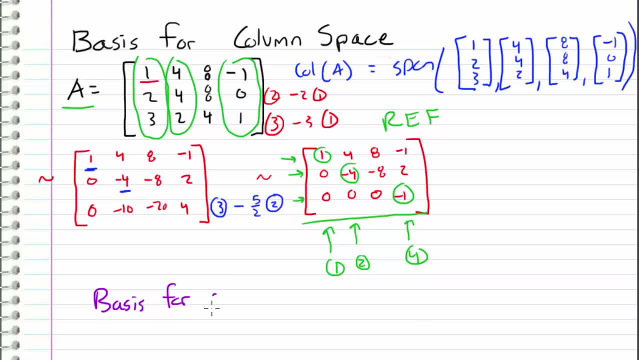 So, in other words, the basis for the column space of A in this example is equal to the set of vectors 1, 2,, 3,, 4,, 4,, 2. And 4. And 4. And 4..